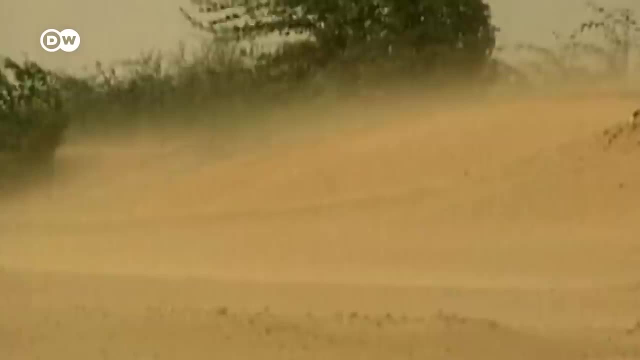 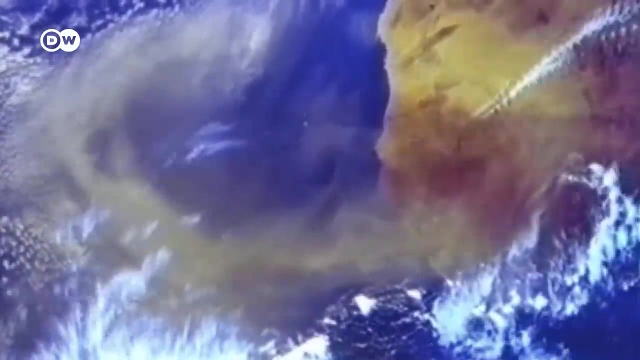 That's half a degree above the previous high set in 2010.. One factor is dust and sand. Global warming has weakened trade winds from the Sahara Desert in Africa, So there's less dust from the Sahara being deposited on the surface of the ocean. 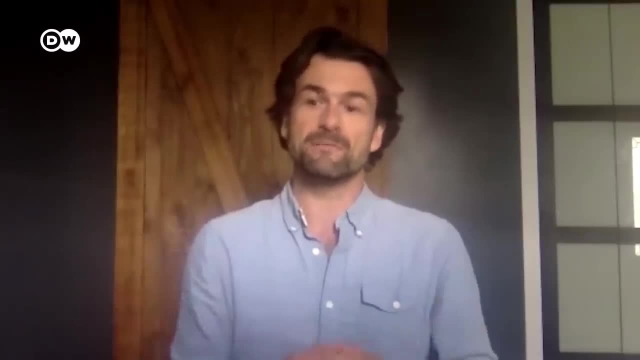 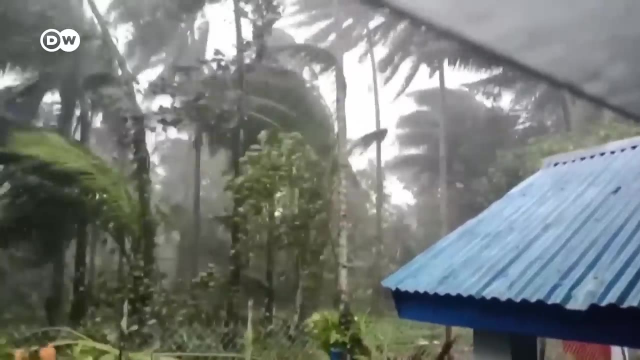 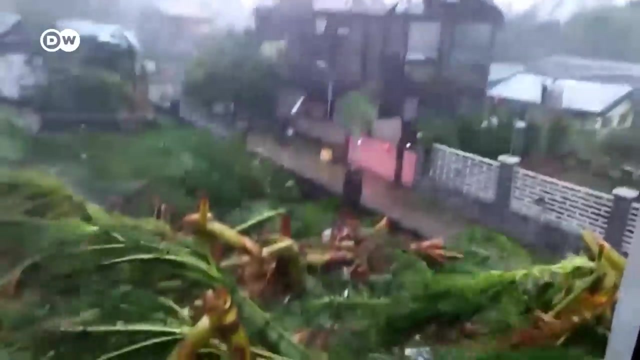 And this, this dust, used to have a cooling effect because it reflects solar radiation back to space. On top of that, El Niño is now officially underway. El Niño is a natural climate pattern that happens on average every two to seven years. It fuels tropical cyclones and boosts rainfall as well as flood risk. El Niño is happening while the world's oceans, pretty much everywhere, are warm, warmer than average. That's not normally something that we see. Those warm waters, combined with El Niño and an already hot atmosphere, are expected. 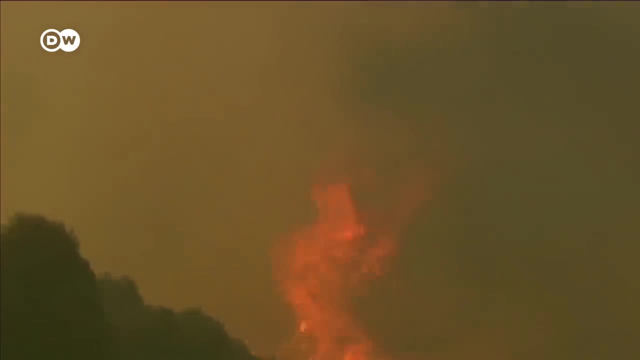 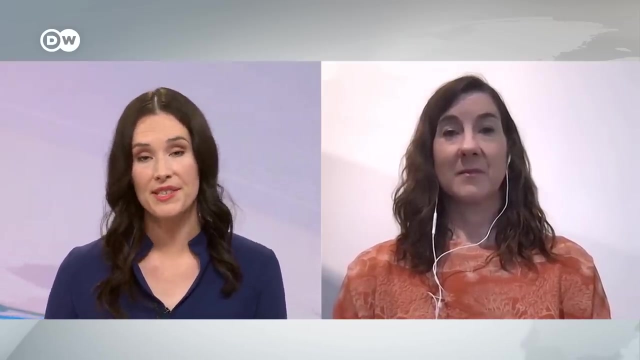 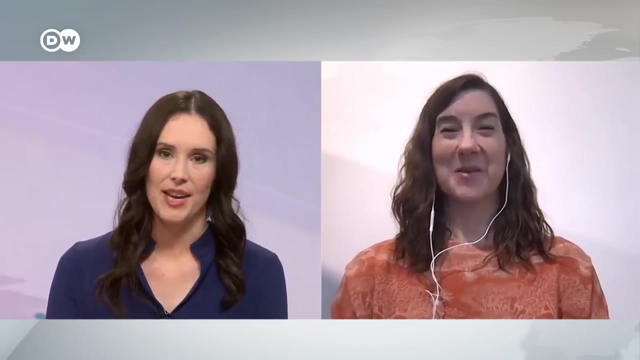 to bring record temperatures to the world this year. Let's speak now to Samantha Burgess, a deputy director at the Copernicus Climate Change Service. It provides the EU with information about climate change. Welcome. We do know that oceans go through natural cycles of heating and cooling. What makes this latest? 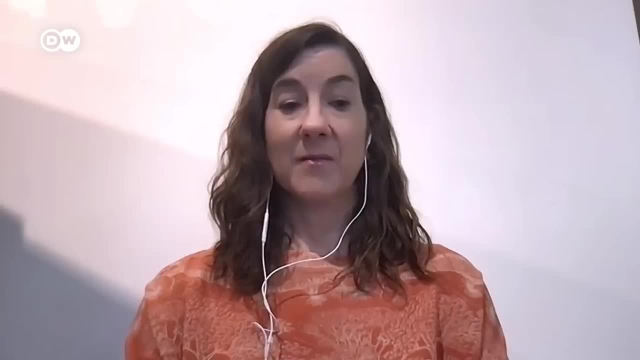 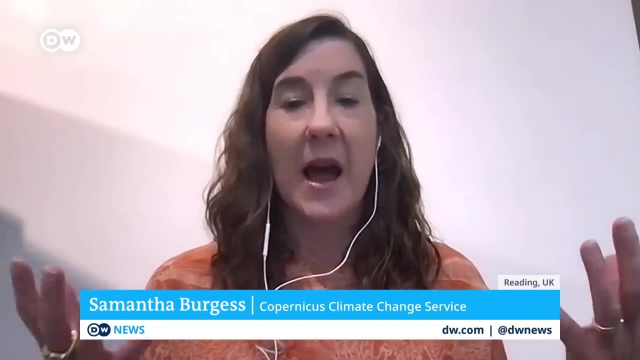 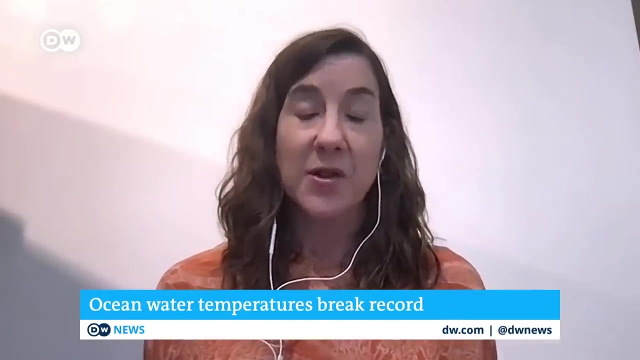 temperature rise so alarming. Hi there and thank you. Yes, so there is an annual cycle in the climate of our planet, both the land temperatures and the ocean temperatures, and normally the maximum ocean temperatures are in August in the Northern Hemisphere summer, but we're seeing very high ocean temperatures. 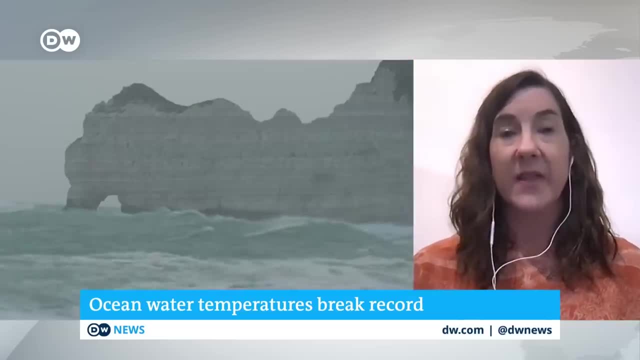 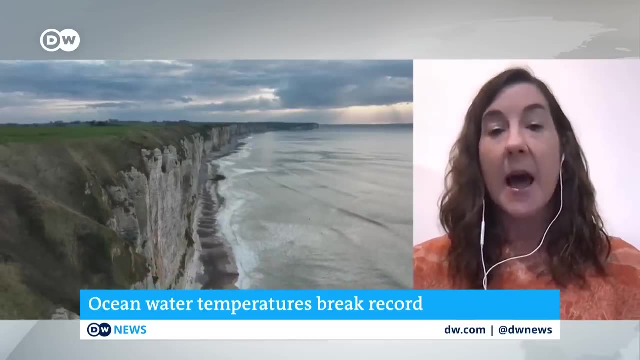 at the moment, in early June, and much higher than what you would normally see for this time of year. In addition to that, particularly in the North Atlantic region, ocean water temperatures are much higher, which suggests a marine heat wave. There are five different. 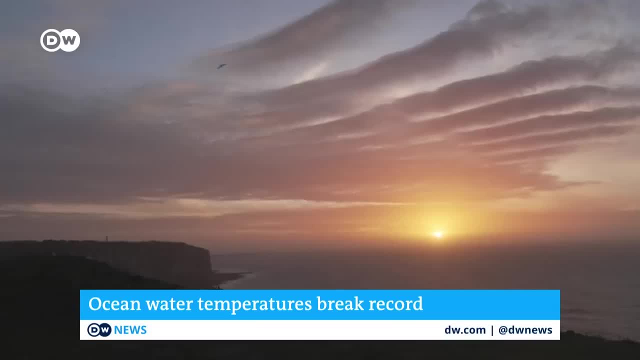 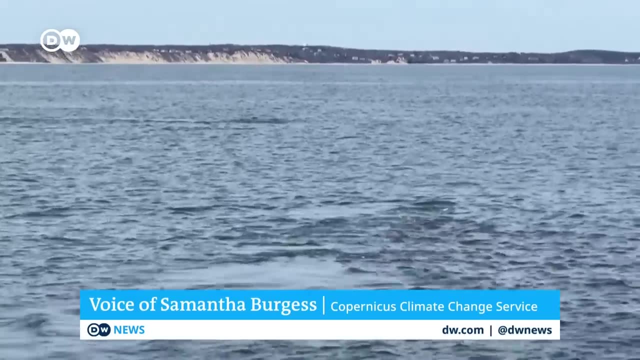 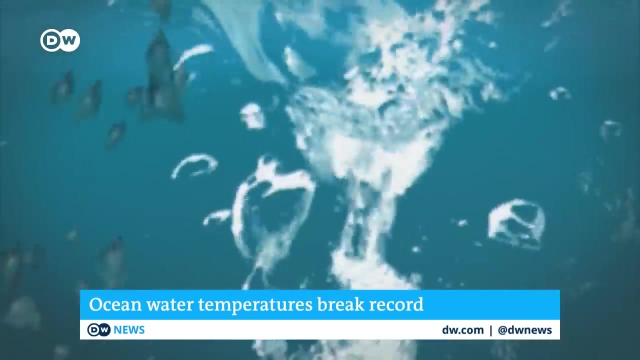 categories of marine heat wave and we're already at the highest category, category five. So I think it's fair to say that we're in uncharted territory in terms of what we're observing in the ocean temperatures right now. So, with this spike in temperatures in the Atlantic Ocean, who is going to be most affected? 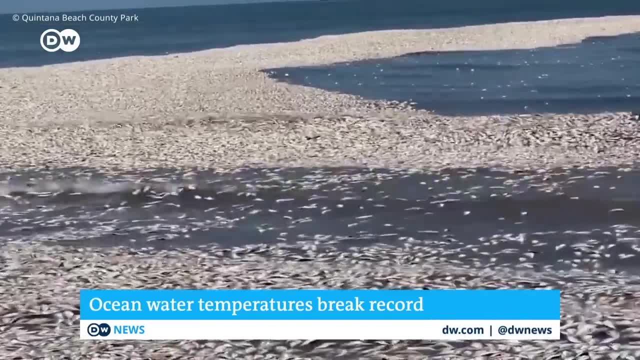 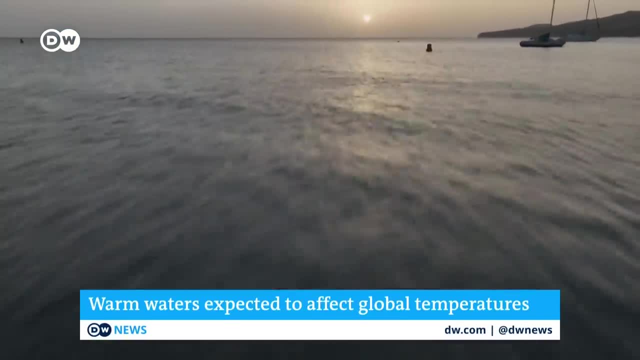 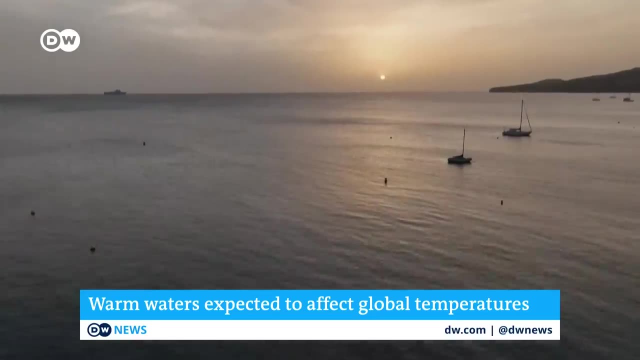 by the consequences. So I think the consequences will play out over a number of months. Obviously it impacts life in the ocean And in your earlier report you mentioned fish deaths. so when the ocean warms up it stratifies So you don't get the mixing between the deep ocean where there's more nutrients and the surface ocean where most life lives. so when you get this stratification, it prevents this mixing occurring and the life in the surface of the ocean quickly absorb all the oxygen and then they don't have the ability to move deeper into the ocean to get new oxygen, so they just die and this happens. 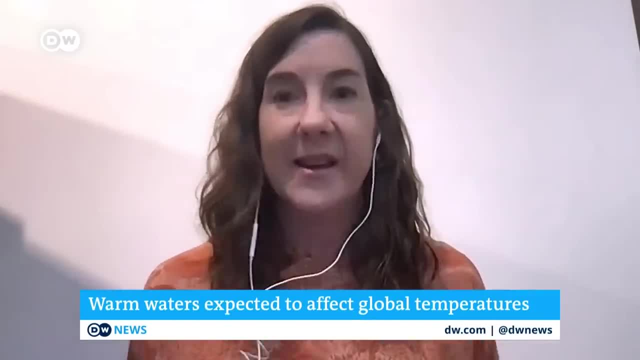 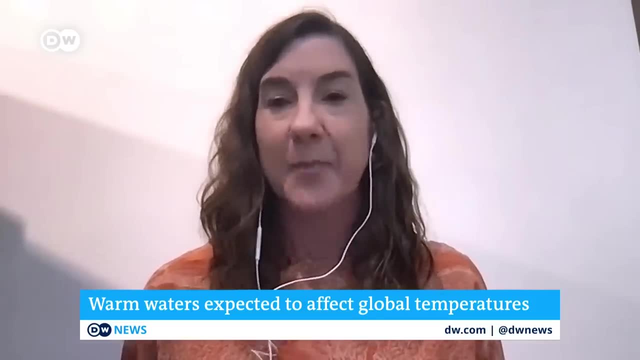 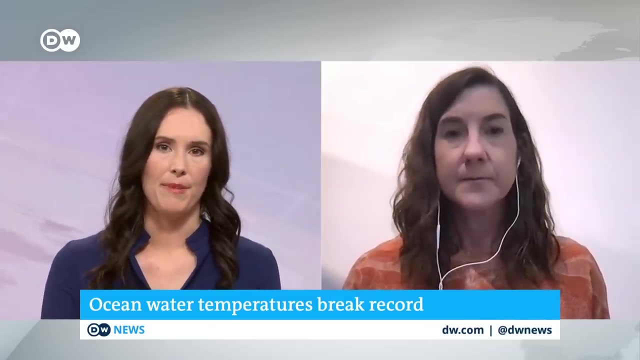 without their awareness, because it's a passive exchange with their gills and, you know, filtering the water. so we've already seen a huge number of fish deaths and the expectation is we'll see more of these. And just explain for our international viewers what is it about measuring the sea. 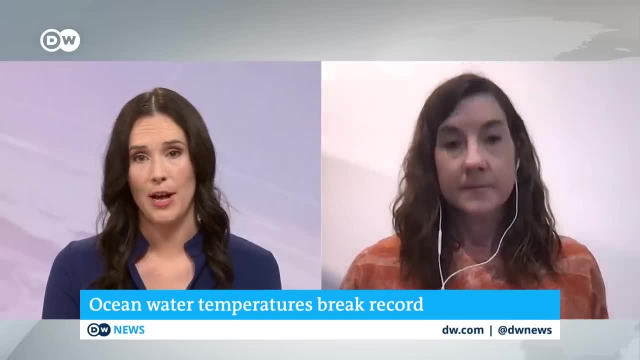 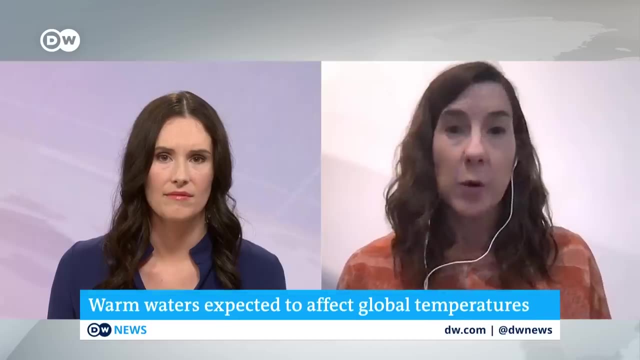 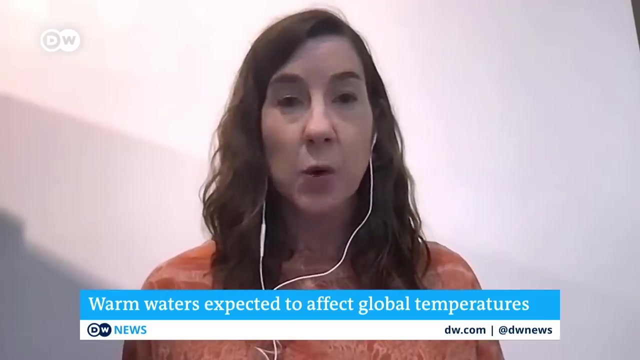 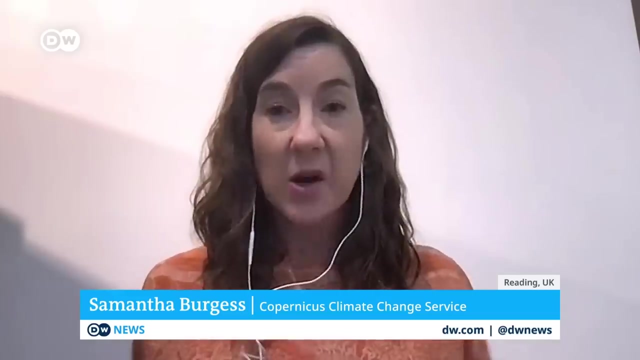 surface temperature. that makes it such a critical metric to help us understand the state of the global climate. The temperature in all forms is a really useful measure of climate change, but we know through science that the ocean's absorbed 90 percent of the excess heat from extra greenhouse gases in the atmosphere. so because the 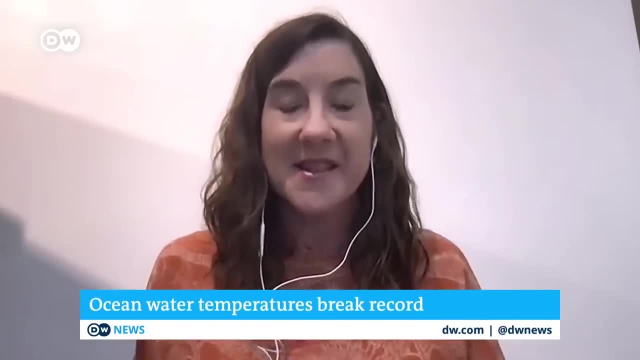 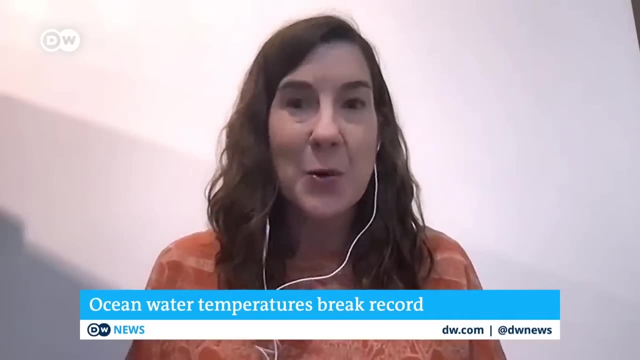 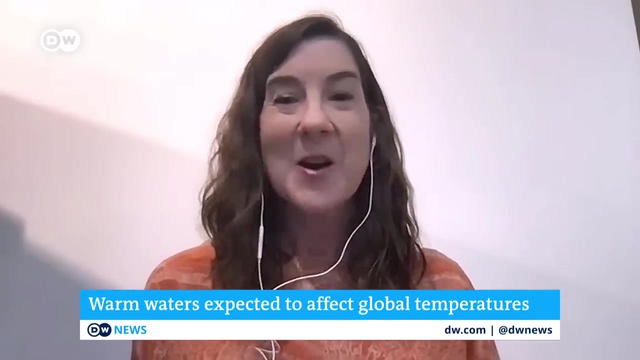 ocean is is the proverbial enormous sponge that soaks up this extra heat. when it gets hotter than what we've seen in the past, it means we don't know what's coming next. so it has implications for life. it has implications for people who depend on the organisms within the ocean. it also has the 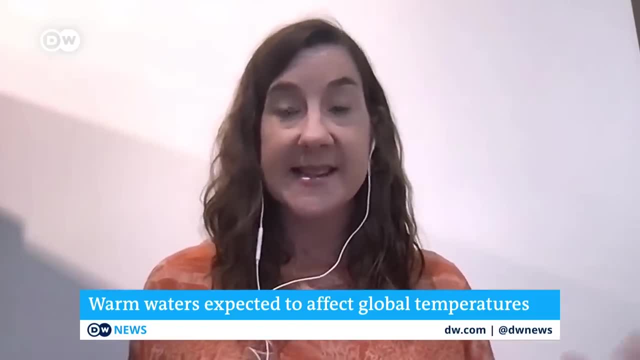 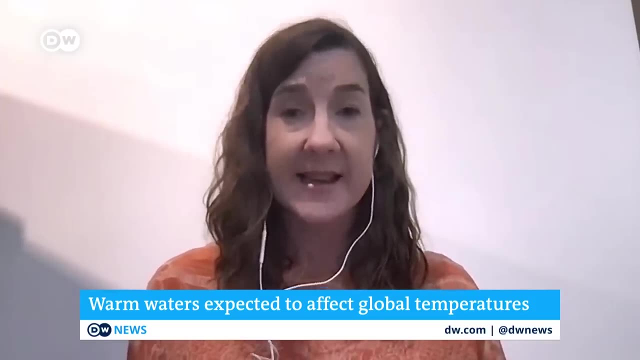 ability to change the climate, So it's a really important measure of climate change. So with high SSTs it's easier for hurricanes to form, for example, so we may see additional storms in the North Atlantic this year and in the other hemisphere and the southern hemisphere particularly. 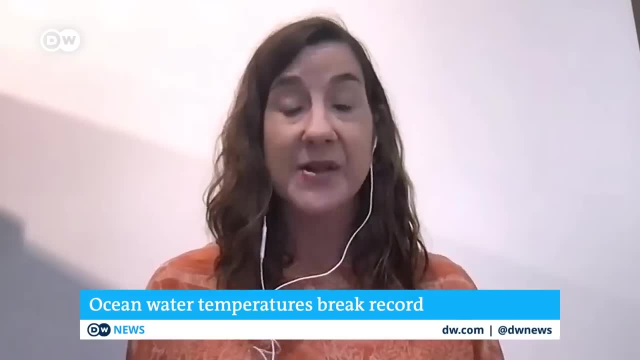 in the Pacific Ocean we also have the developing El Ninos. We have very high sea surface temperatures that formed off the coast of Ecuador and Peru and now they're spiking across across the equatorial Pacific and we're expecting this El Nino signal to happen in the next few years. So it's a really 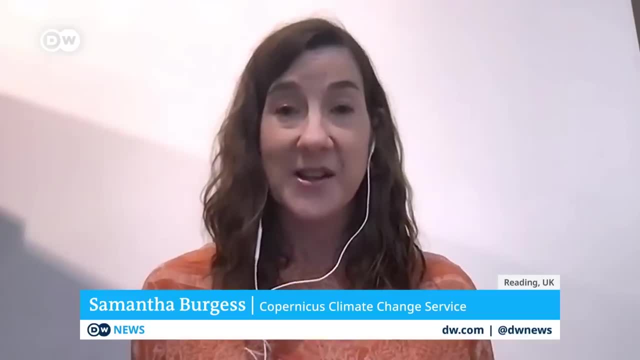 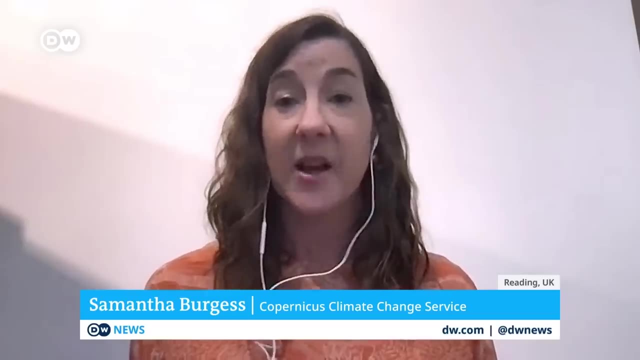 important measure of climate change that we're hoping to continue to develop. We don't know how strong El Nino is going to be, but this means we'll see higher temperatures in the Indo-Pacific later this year, which may also lead to other impacts like coral bleaching, where again, we'll see massive loss.